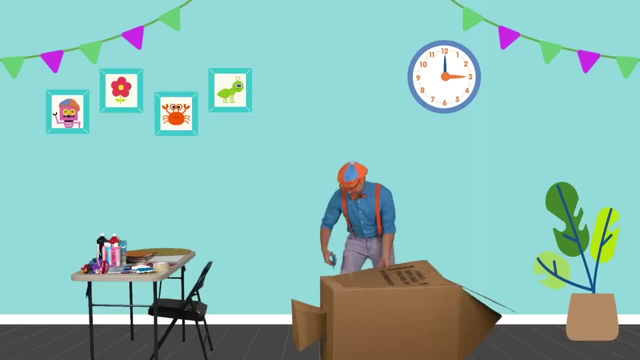 I am using these scissors, nice and safely, to cut a giant window out of it. Whoa, look at that. Wow, Ooh, now I can sit inside it later. Hmm, then we can explore outer space. I am so excited. 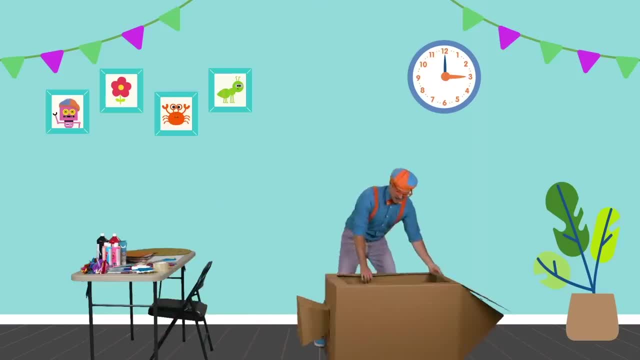 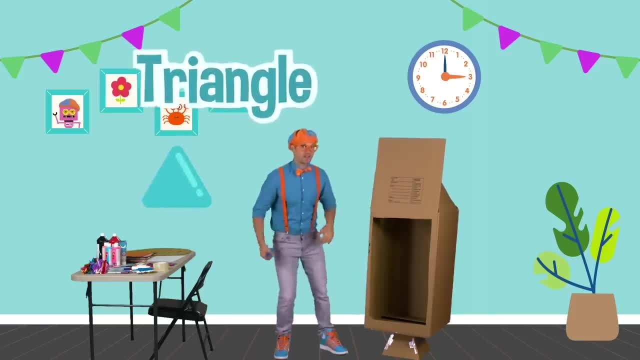 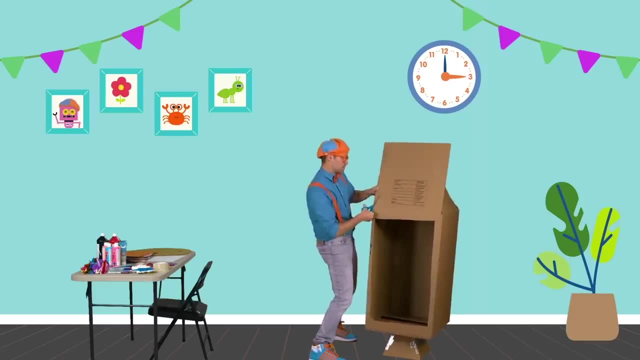 This is a square. This is a square. This is a square. Yeah, but we actually need to make it a triangle. Yeah, But we actually need to make it a triangle. So let's take our scissors. Yup, With your parents' grown-up supervision, you can cut this. 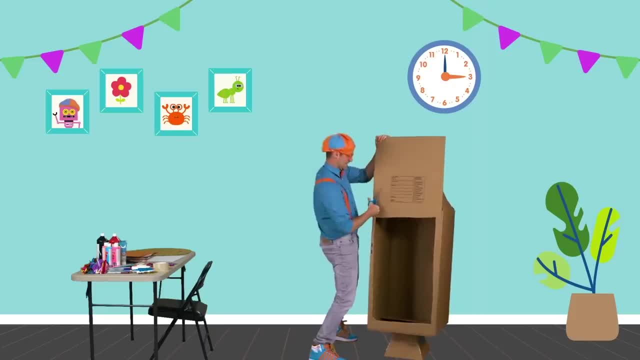 Nice and carefully. Oops, Okay, one side is done And now we need to do the other side. Come on, here we go: Woohoo, Look at that, It used to be a square, but now it's a triangle. Okay, now we need some tape. 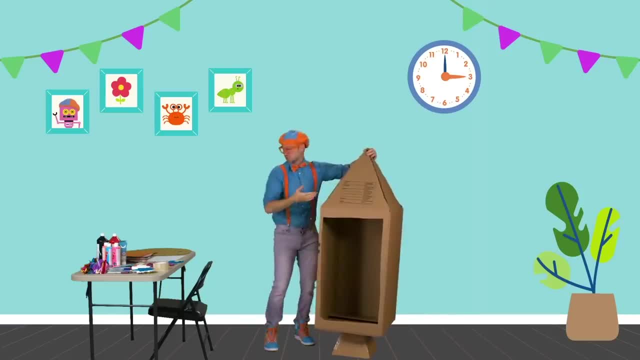 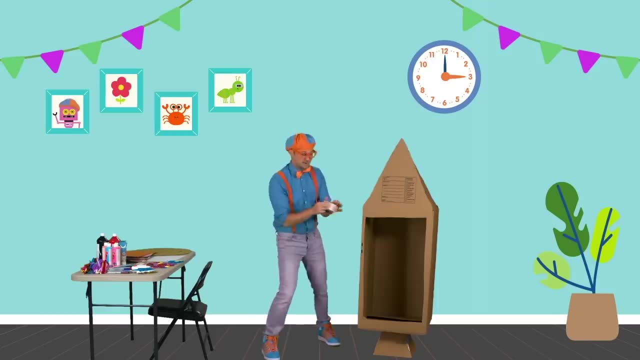 to tape it to make the top of the rocket ship. Okay, here we go. Let's grab the tape, Pull off a big piece of tape, Whoa, Alright, let's give it a little slice. Okay, there we go. 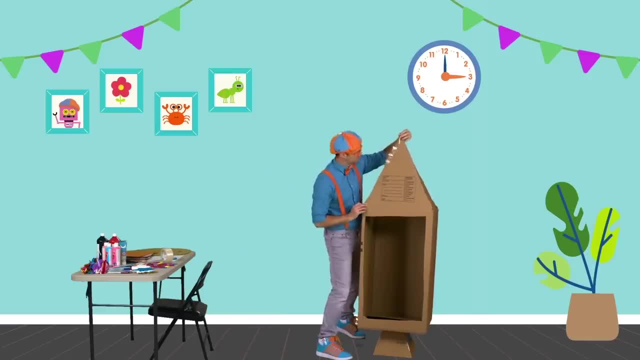 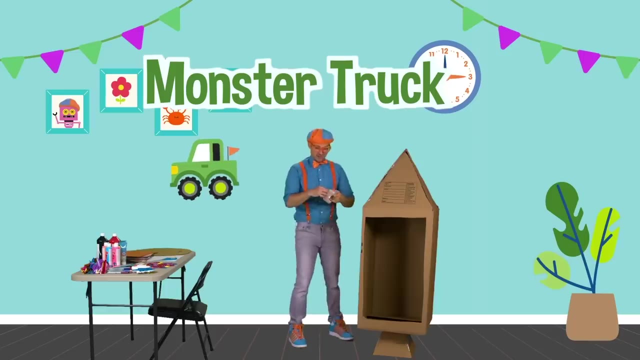 Whoa Put that there. I love making things out of cardboard boxes. You can make so many things. Today we're making a rocket ship, but one time I made a monster truck. Another time I made a dolphin And I named that dolphin. 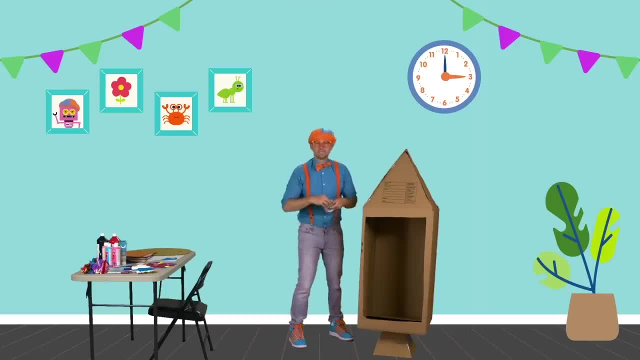 What was that name? I think it was Dolphy Whoa. Sometimes the tape gets stuck, but that's okay, We got it. Alright, There we go. Give it a little slice And then tape up the other side. Wow, Here we go. 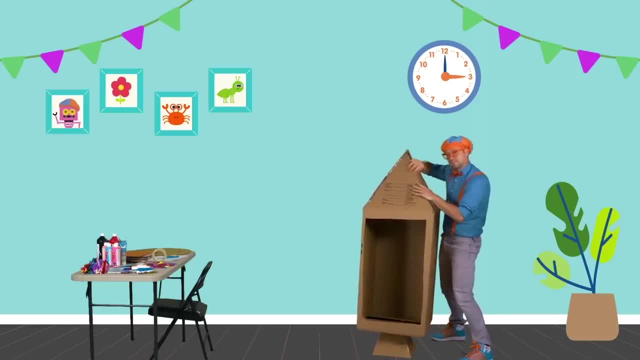 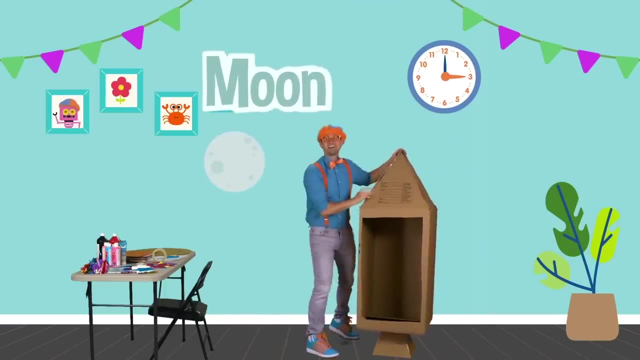 I am so excited to go into outer space. Have you ever seen the stars at night? Yeah, they're so bright. And the moon- I love the moon. Have you noticed that the moon sometimes is a full moon? Yeah, sometimes it's a half moon. 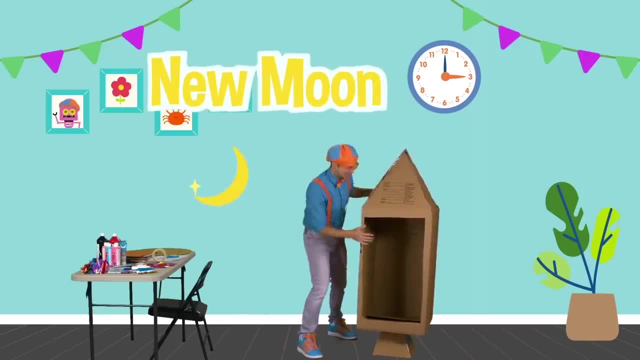 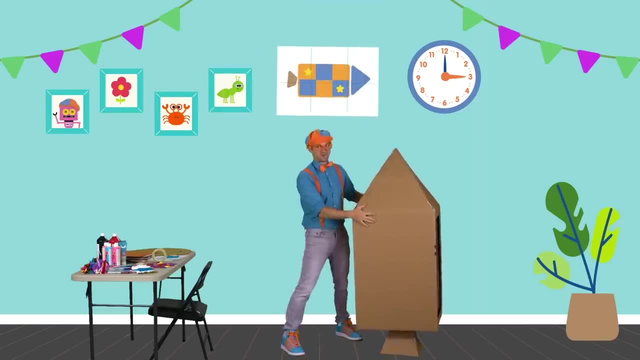 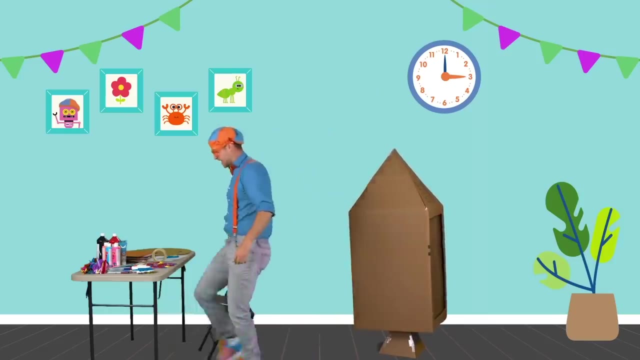 And sometimes it's a new moon. Okay, let's give this a little twist. Now it's time to design our rocket ship. I am so excited. This is one of my favorite parts. So the first step to design is to have a plan. 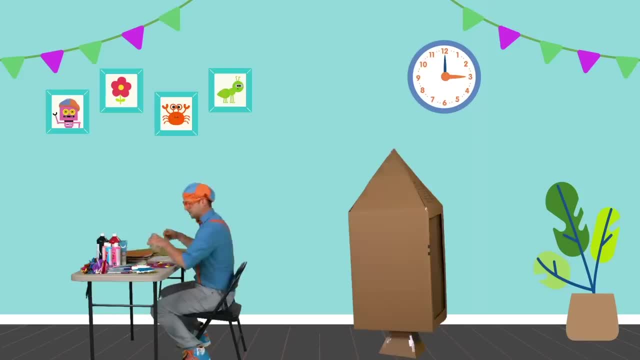 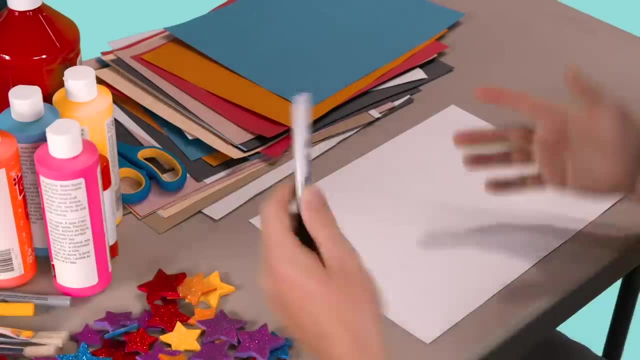 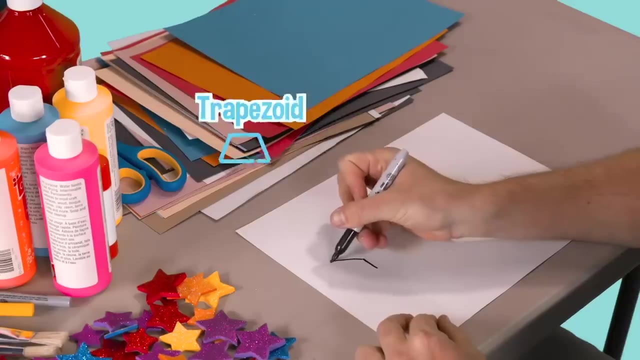 Let's take this white piece of paper right here and let's draw the rocket ship. So the first thing you need to do is plan- Plan how the rocket ship is going to look. So let's draw the rocket ship. So we have a trapezoid over here. 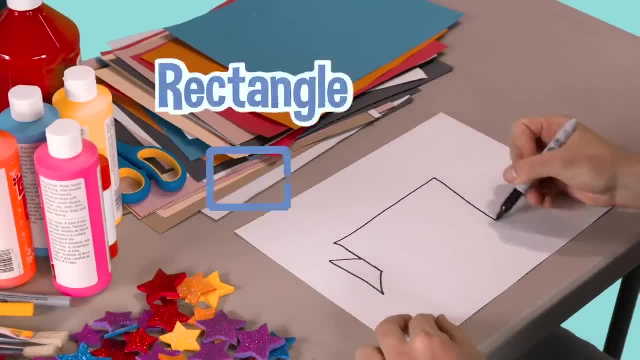 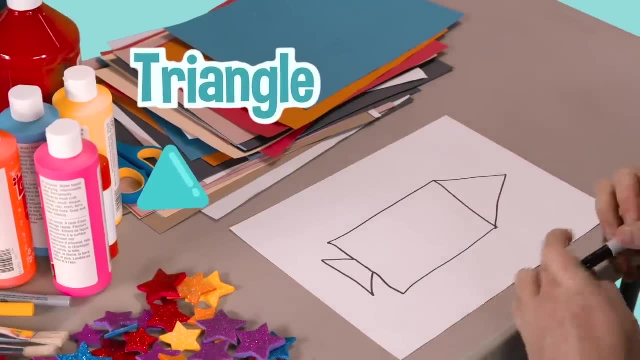 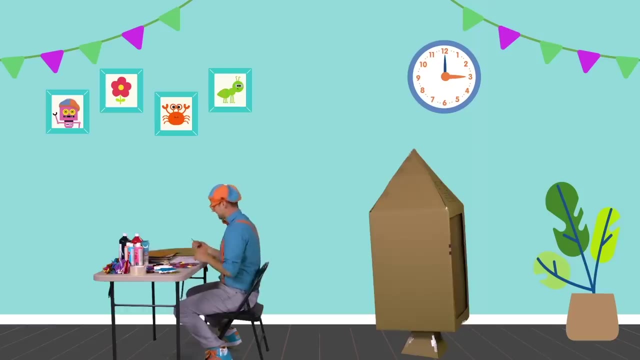 Then we have a big rectangle for the body of the rocket ship, Then we have a triangle for the cone of the rocket ship And obviously I want a lot of color. So first let's take some orange. Perfect, I love orange. 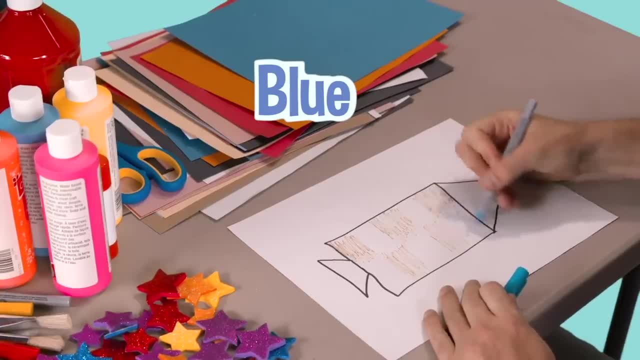 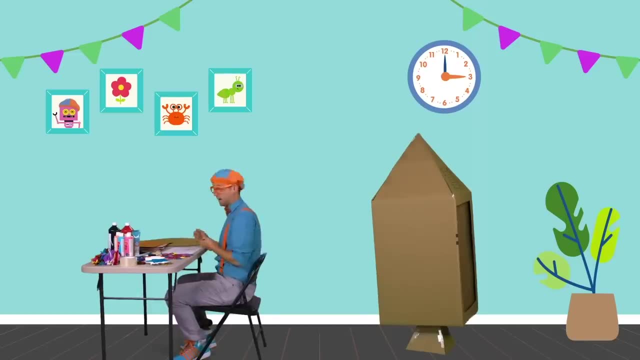 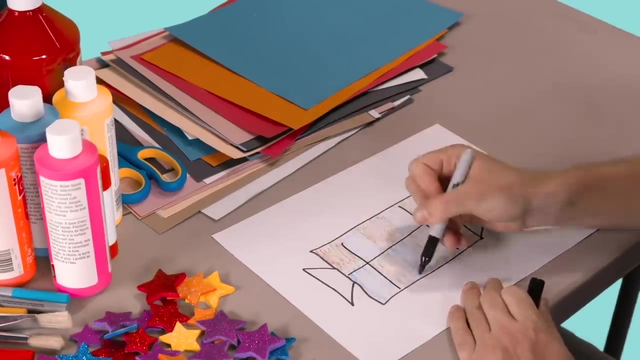 Then let's take some blue, Let's color it in. I have a plan. I'm going to use colored paper for that. So I'm actually going to use this black marker to symbolize that these are pieces of paper. Let's do that later. 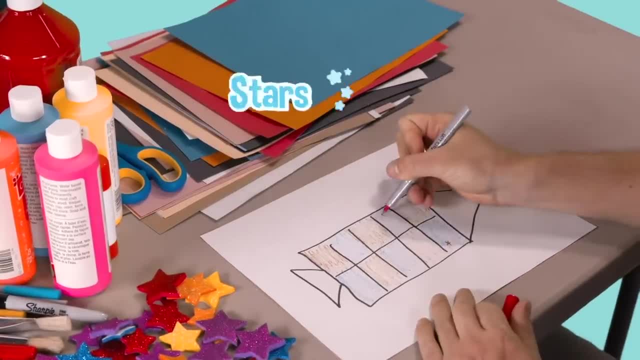 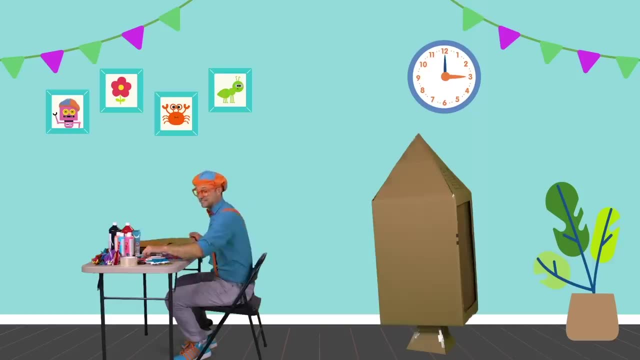 There's a lot of stars here, So let's actually make some stars right here. Yeah, I love stars Because you see them at nighttime when you look up in the sky and they twinkle Kind of like Twinkle, twinkle little star. how I wonder what you are. 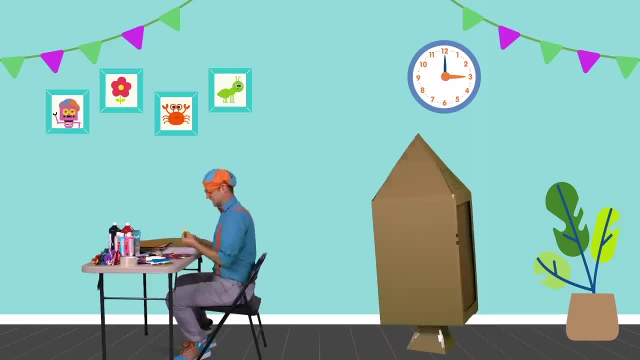 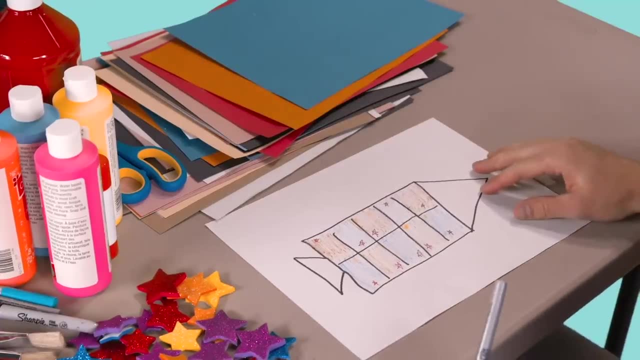 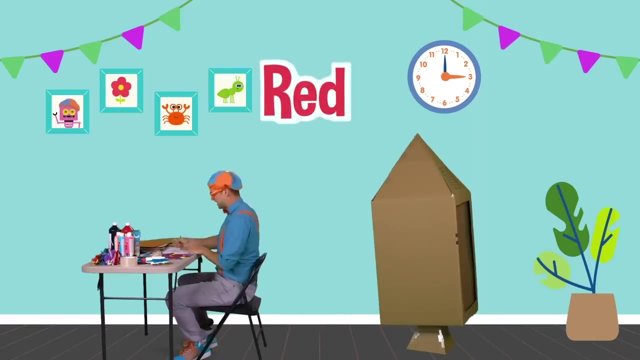 You know that song. I like that song too. Hello Yeah, That's a beautiful color. Wow, Our rocket ship is looking so good. Alright, I think I have a really good idea. Let's take the color red, Because it's nice and bright, And spell my name. 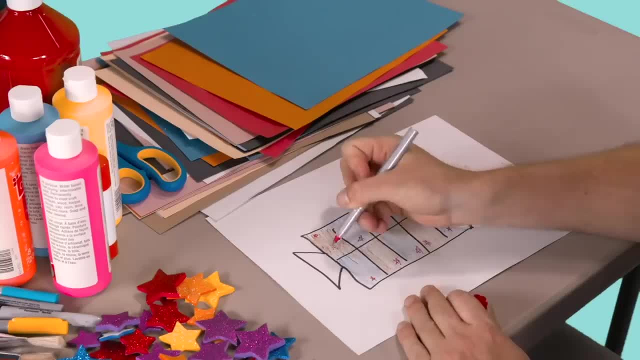 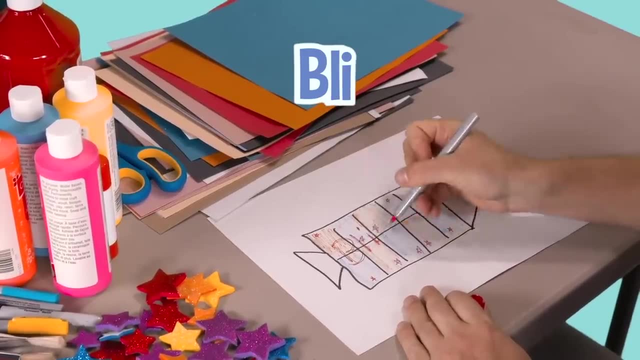 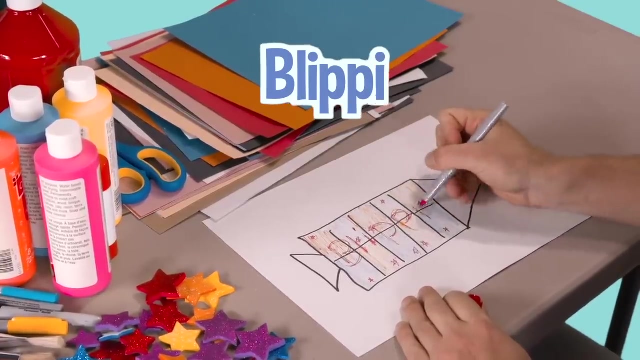 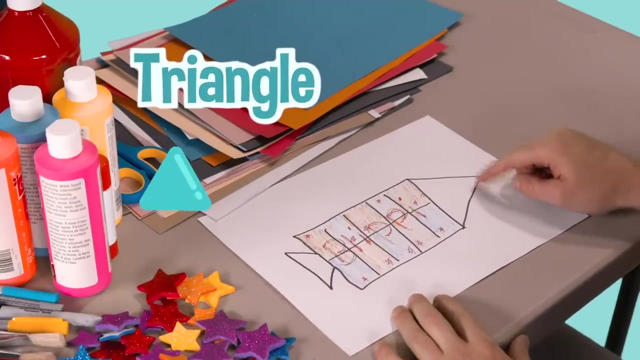 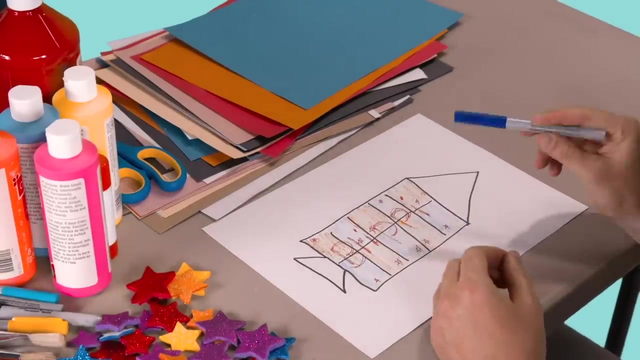 Will you spell my name with me? Ready B, L, I, P, P, I, Blippi, Perfect, Alright, So that is the plan. Looks like this triangle, The top of the rocket ship. Yeah, We could color it. How about we color it? yeah, blue. 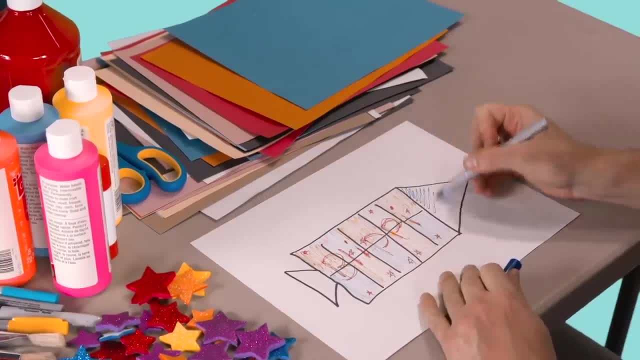 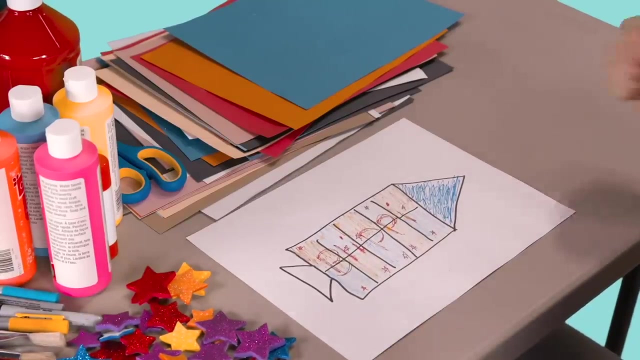 I like blue And we actually have a lot of blue paint on here, So we can actually just use blue paint for this part. Wow, Perfect, Wow, I think. if we can make this rocket ship in real life, it's going to be so good. Alright, Here we go. 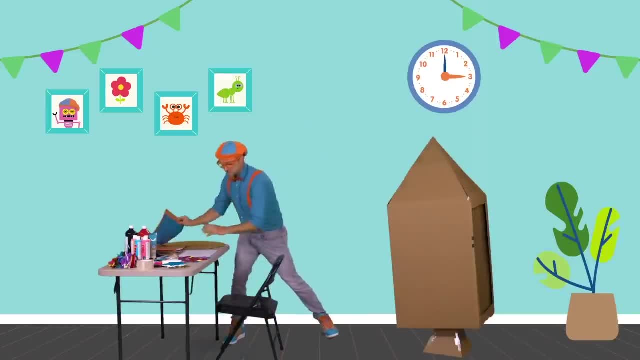 Alright, Like I said, first thing we have to do is use the blue and orange colored paper to put on the side, Just like this. So let's take the glue stick. Yeah, Yep, Put a lot of glue right on the backs. 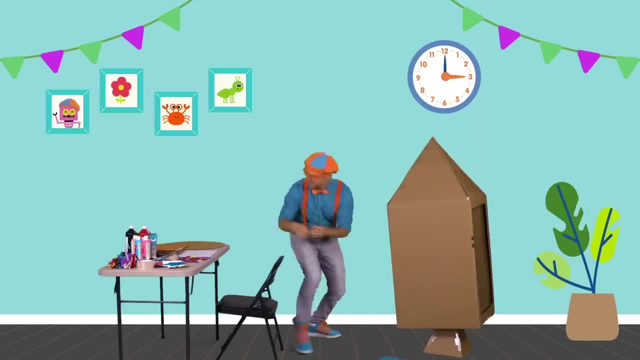 Just like that. Okay, There's two pieces, Okay, There's one, And here's the second piece. Alright, There's one, two pieces of paper And we got to do two more, Yeah, Which will make one, two, three, four pieces. 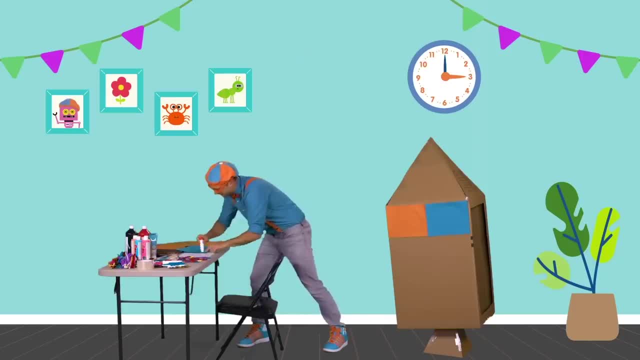 of paper. I'm going to put the glue on them right over here. Okay, Now we have four pieces: One, two, three, four. Okay, Now we have four pieces: One, two, three, four. Okay, Now we have four pieces: One, two, three, four. So let me finish. 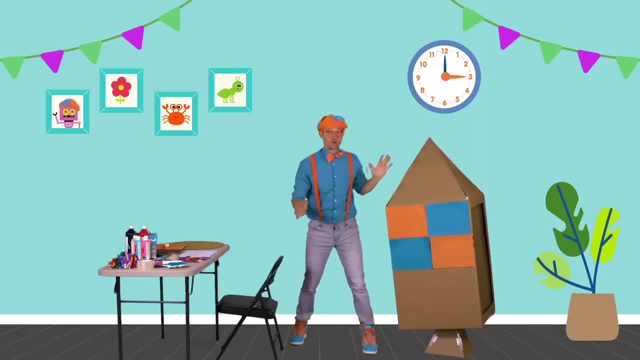 the rest, and then we'll see how many we have in total. after I'm all done, Alright, Whoa, It's falling apart. Well, sometimes if things fall apart, you just have to fix them. Okay, Here we go, And after we fix this, then 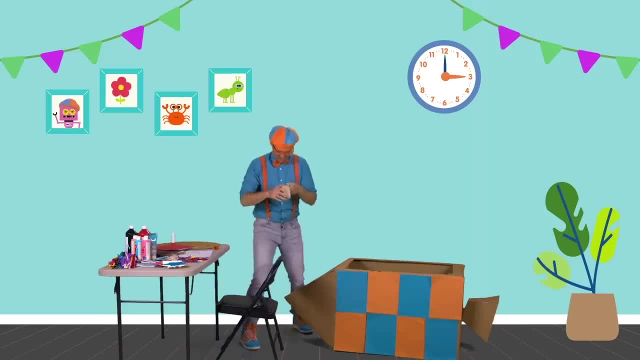 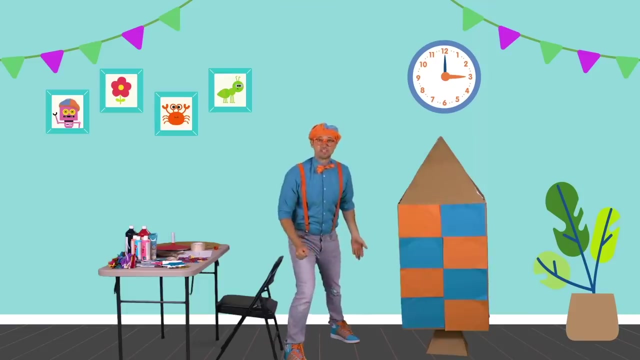 we can count all of the colors, So let's take our tape. Alright, Now the rocket booster is all fixed. Yep, There we go. Okay, Now let's count all of the colored pieces. Yeah, The blue and the orange pieces. Those are my. 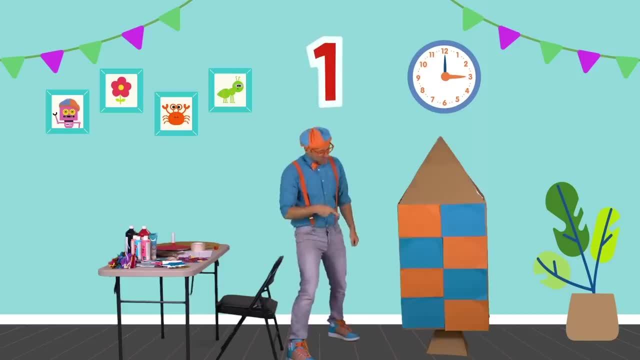 two favorite colors. Okay, There's one, two, three, four, five, six, seven, eight, Eight pieces of paper. Good job, Okay, What else did we have on our piece of paper over here of our initial plans of our rocket ship? 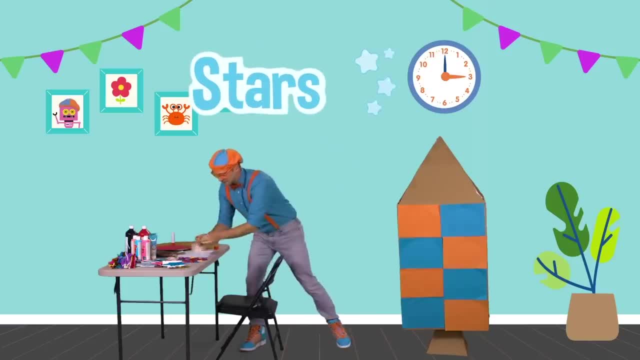 to go to outer space. We had stars. Yeah, Remember We had yellow stars. Yellow star, Another yellow star. Wow, They're so bright and they twinkle just like the real thing. Okay, And let's put some blue stars on there. 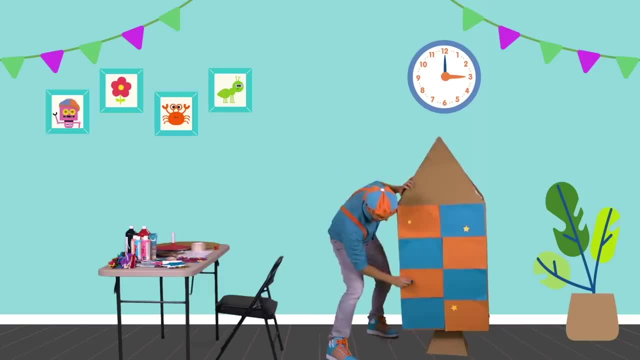 Can you think of anything that's the color blue My shirt. What about the big, vast blue ocean? Yeah, Here's another blue star. There we go. What about a purple star? Yeah, I like the color purple, Right there. 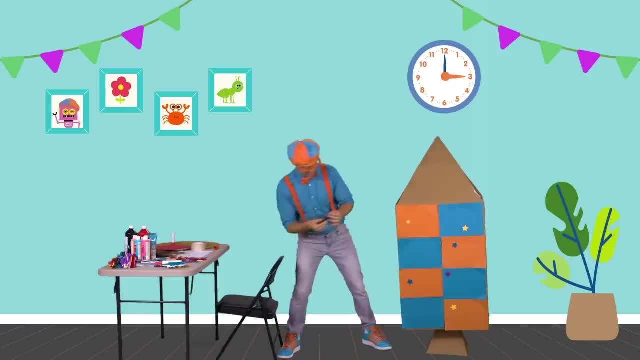 And last but not least, another purple star Right there, Perfect, That looks so cool. Alright, So, as you remember, we have to spell my name on it because that's what was on the plans. But before we do that, let's. 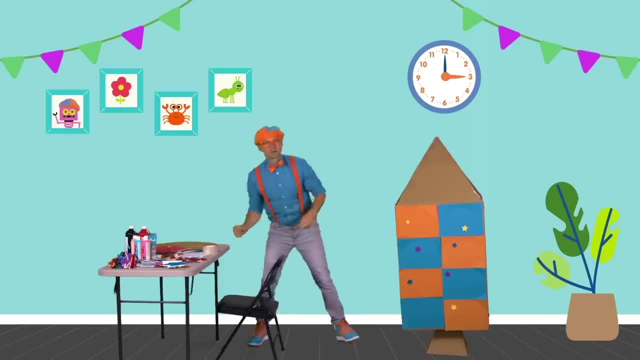 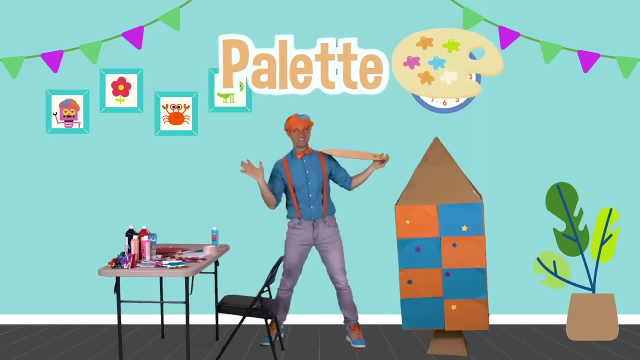 do the top of the rocket ship. Remember what color I said I was going to paint it? Yeah, The color blue. Okay, Let's take some blue paint and my painter's palette- I'm an artist- And let's take a paint brush. Ooh. 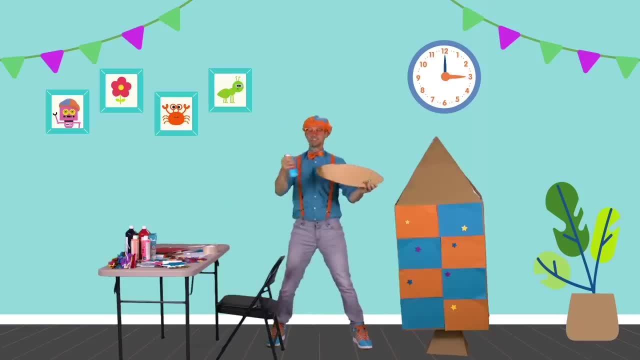 I love painting. Okay, Let's squeeze some blue paint right on top. Whoa, Whoa, Whoa, Whoa. That's so much fun. Okay, Let's give it a little dab. Let's do some painting. There we go, Wow. 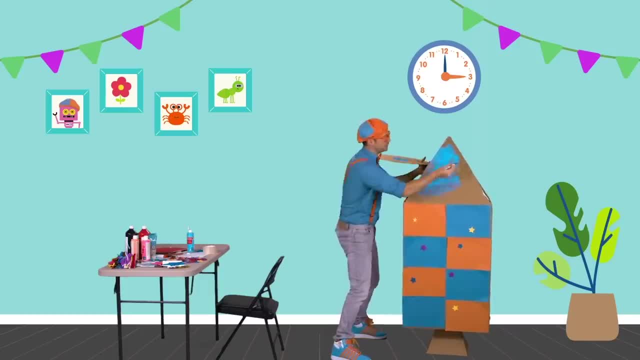 This is such a pretty blue. Wow, Whoa, Whoa. There we go. Have you ever used paints before? They're so fun. You can use a paint brush and you can even use your fingers sometimes. We won't do that today. 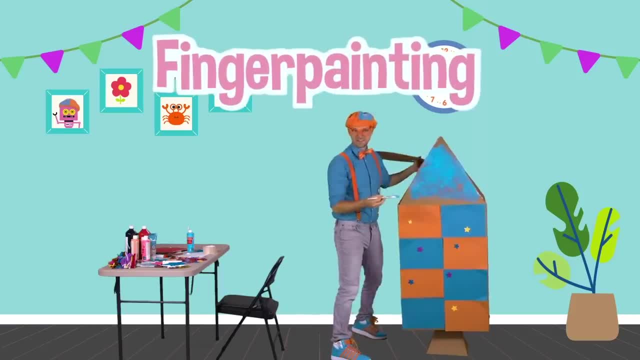 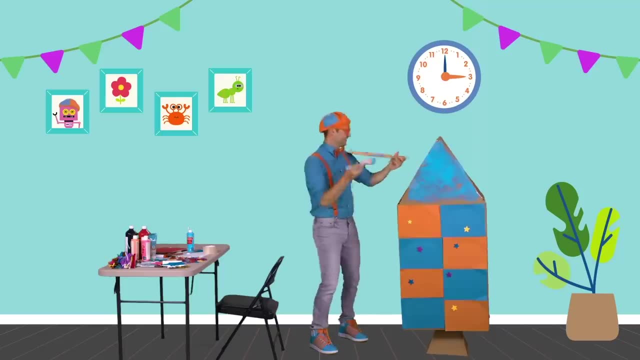 But that art technique is called finger painting. There we go. How does that look? Do you like that? Yeah, I do too. Okay, Let's put this away. You need to stay nice and clean and organized. There we go, And. 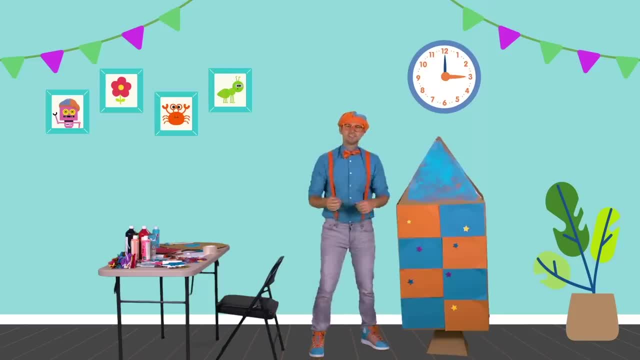 remember the last thing we needed to do. We needed to spell someone's name. Oh yeah, My name Blippi. Will you spell it with me? B-L-I-P-P-I, Blippi, Good job, And do you remember what color? 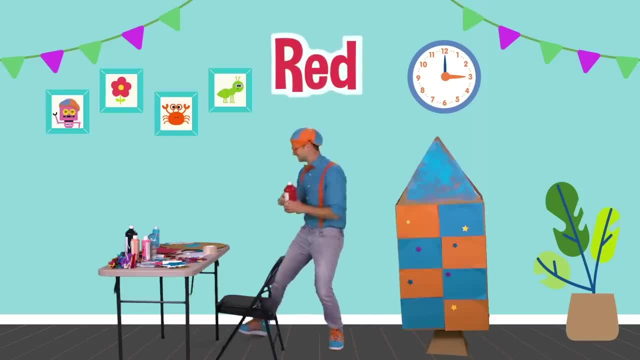 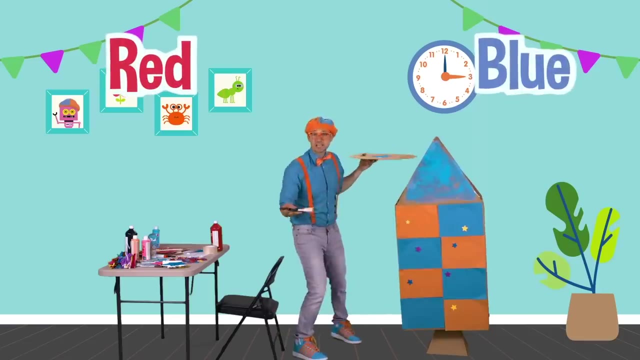 Yeah, The color red. Okay, So let's use a new paint brush, Yep. And then we need to make sure we don't mix the red and the blue, Because then it won't be red anymore And it won't be blue. 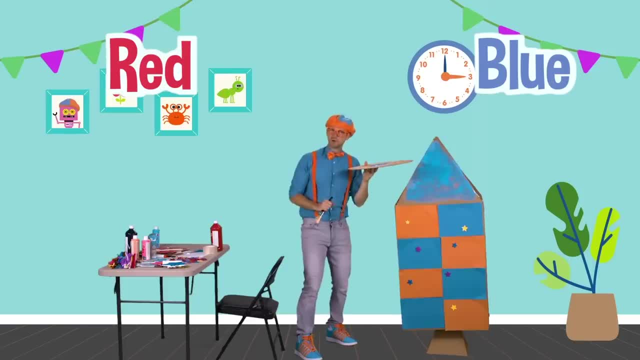 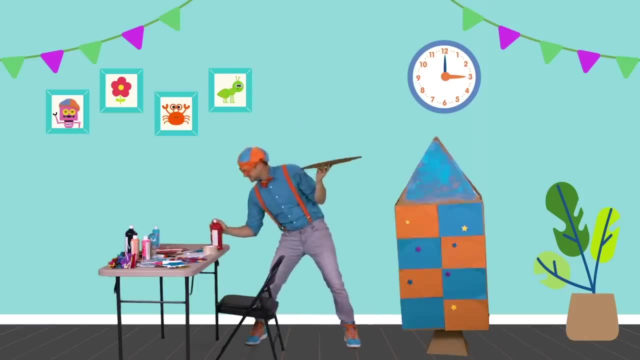 Do you know what color you get when you mix blue and red? Yep, Purple, But we're going to keep them separate, So let's take this cap off. Oh, There is so much paint in here And I like to use a lot of paint. 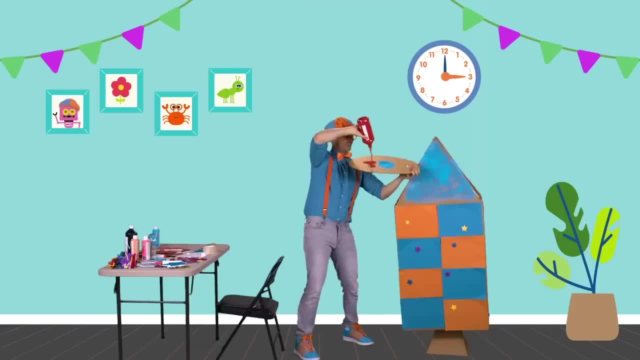 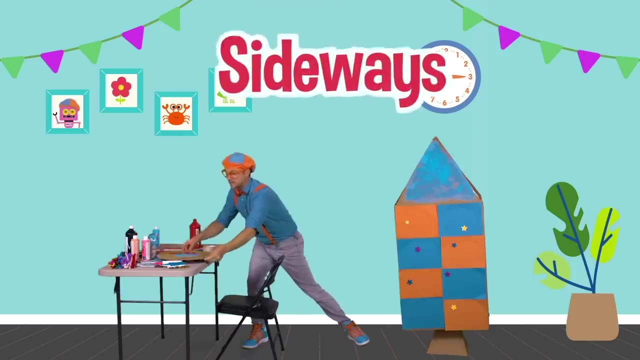 Whoa. Oh, There we go. Wee, Wow, A little bit more. Alright, There we go. Okay, Let's, before we paint it, we should probably lay it down sideways, because we need to write my name, which is sideways. 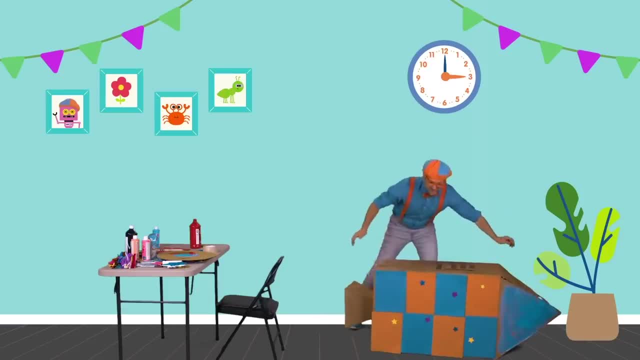 Yeah, There we go Like that. That's how we write Sideways. Okay, Let's take our paint brush and let's put the letter B right here. Alright, Now that we have the letter B. the second letter is the letter L. 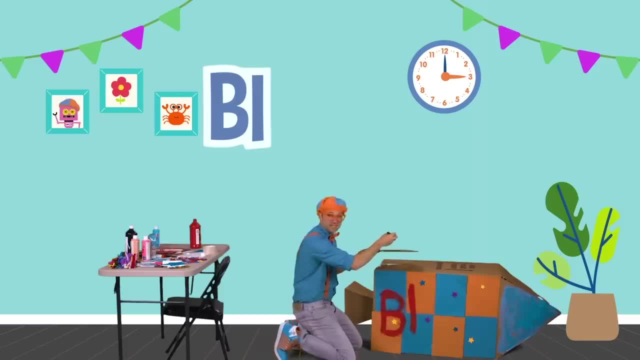 Yeah, Just like that. The third letter is an: I Ready, Okay, There we go. B-L-I. You know the next letter: A P, Yeah, B-L-I P, Alright, B-L-I P, P, Yeah, Here we go. 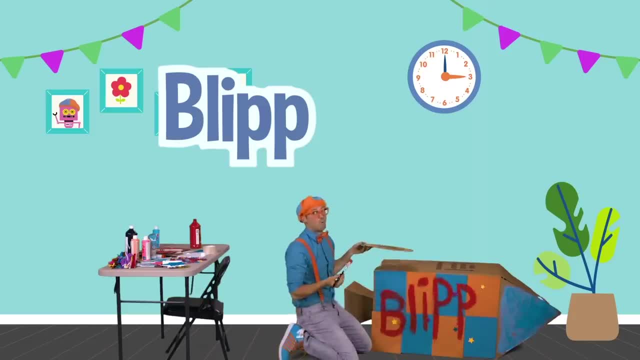 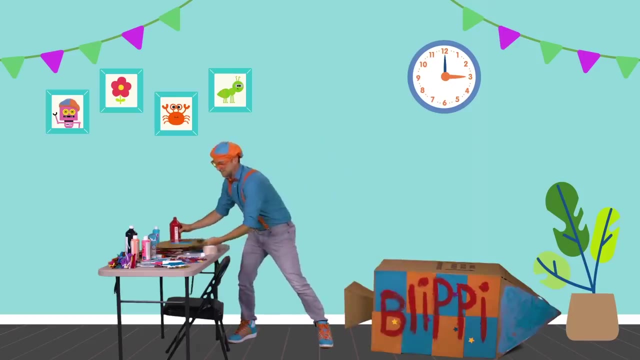 Alright, Alright. One last letter: B-L-I, P-P-I, B-L-I, P-P-I. Blippy, Good job, Blippy, Good job. There we go. We just completed the rocket ship, So now we got to get inside. 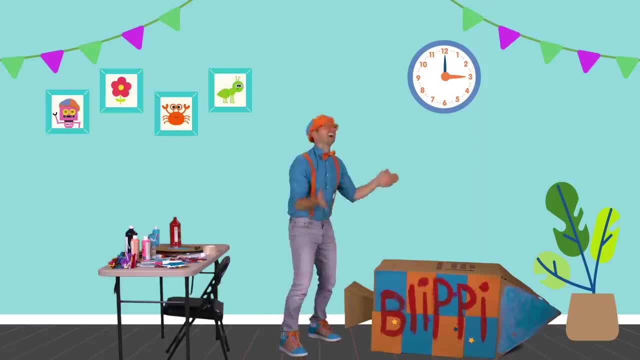 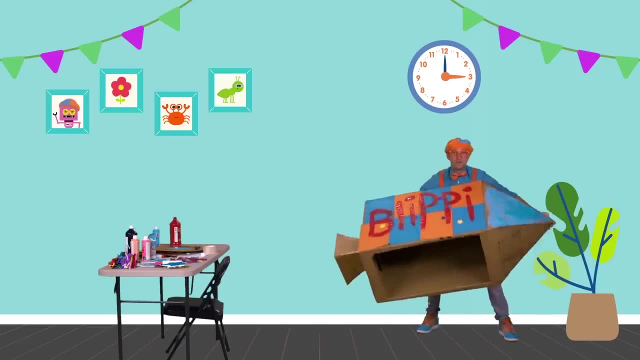 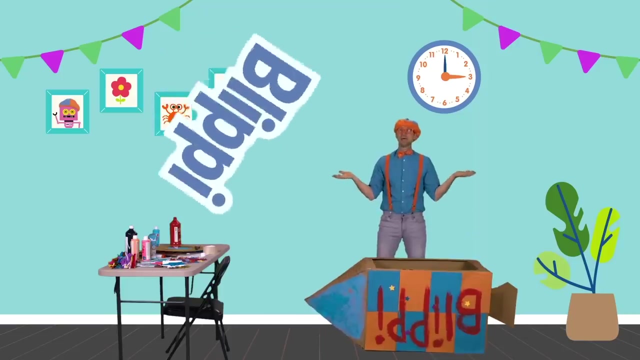 Oh no, Do you see what I did? We're so silly, We're so silly. Check this out. The window is right there. Yeah, That means we have to twist it this way. See, And now my name is upside down. 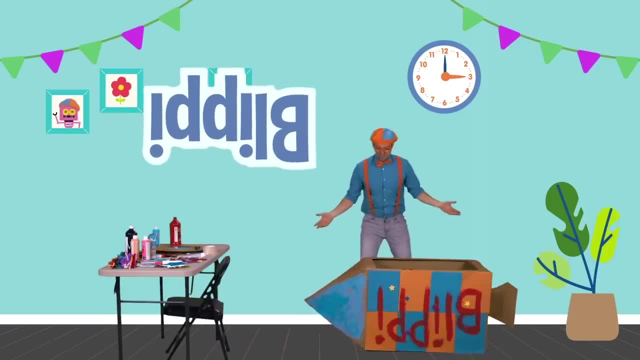 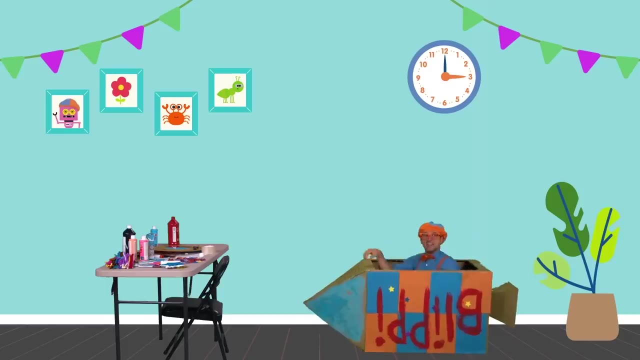 That's okay, though We're going to fly through outer space in this new cardboard rocket ship. I am so excited With my name being upside down. So silly. Are you ready, Because I sure am? Here we go, Whoa. 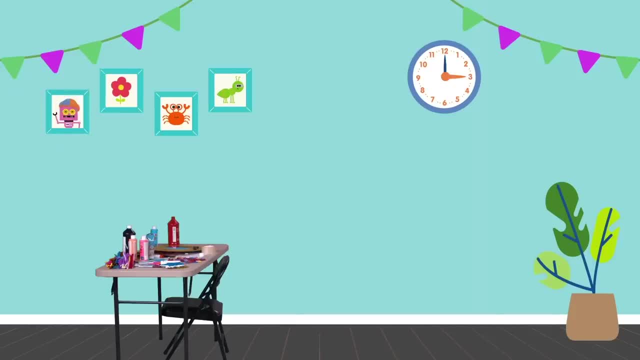 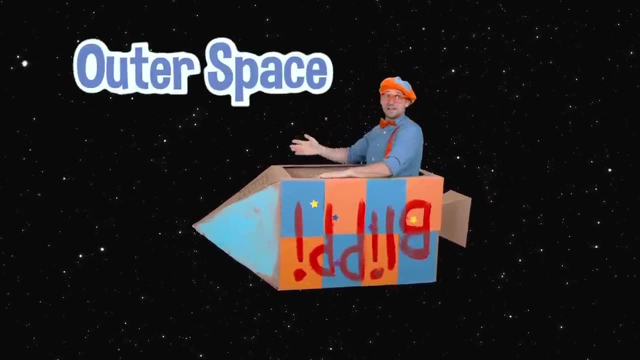 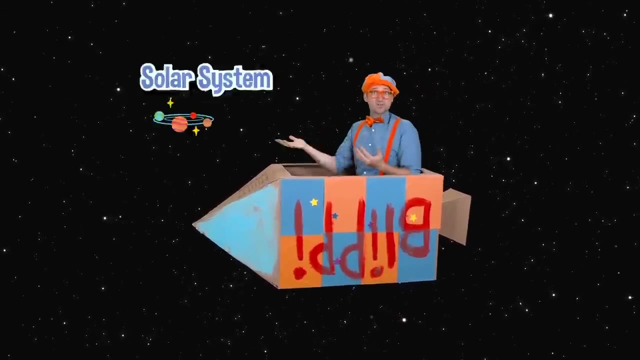 Whoa, Whoa, Whoa Woo. Hey, I love outer space. Good job building the rocket ship with me. Now that we're in outer space, I think we should explore our solar system and learn all about it. All right, Here we go. 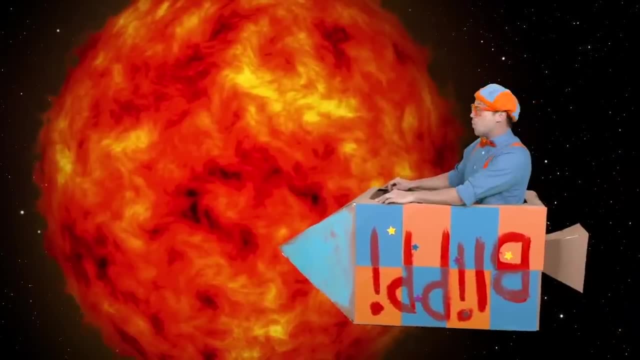 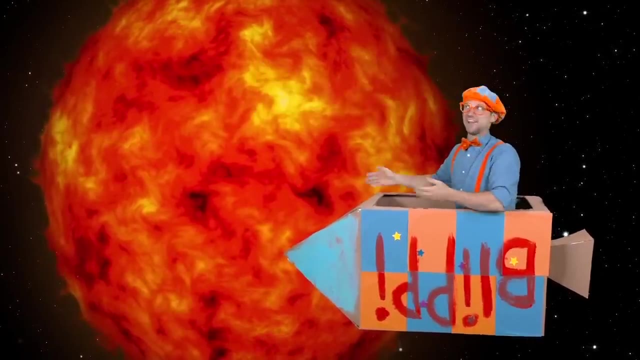 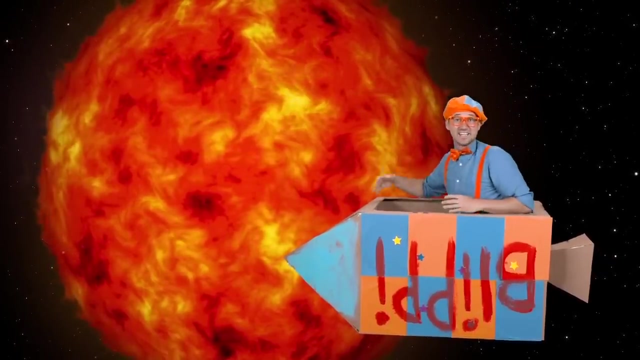 Whoa, Whoa, Whoa. Look at that. That is our sun And its name is called the sun. How original. Our sun provides all the light in our solar system, And that light takes eight minutes to reach the Earth. 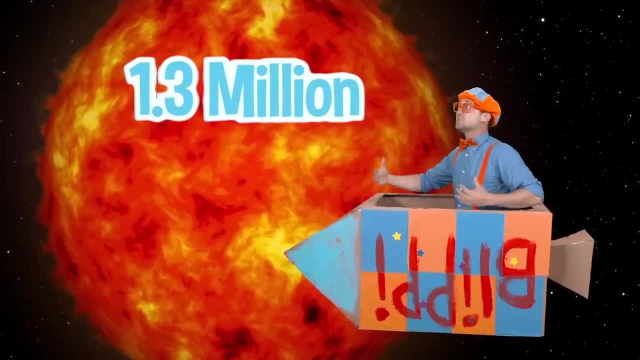 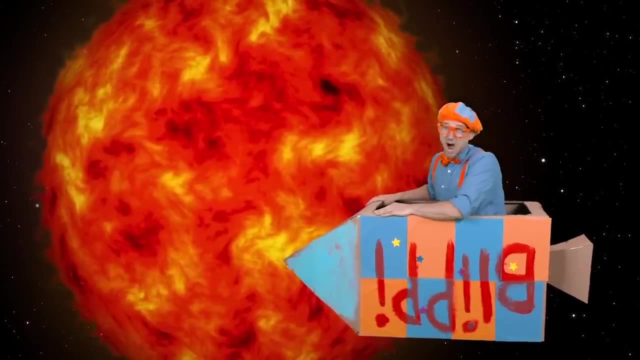 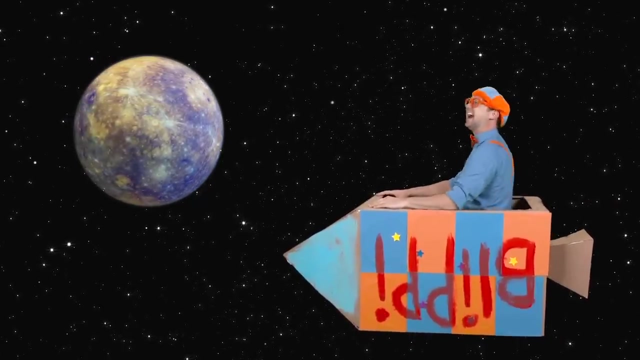 And the sun is so big, There's 1.3 million Earths that can fit inside of it. Whoa, That's a lot of Earths. Here we go, Whoa, Whoa. Outer space is so much fun. 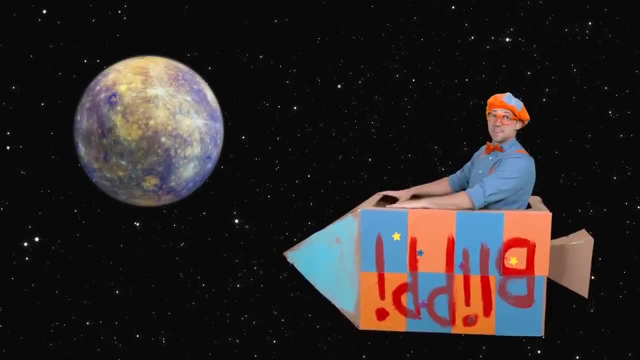 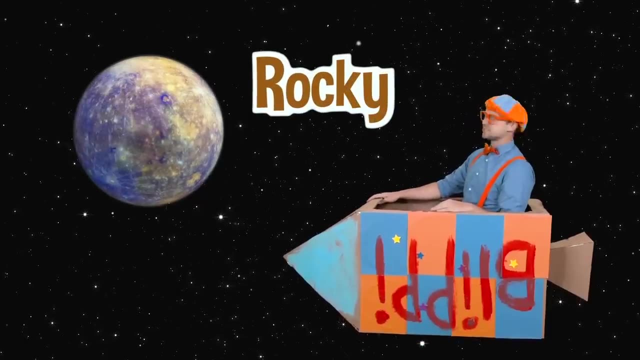 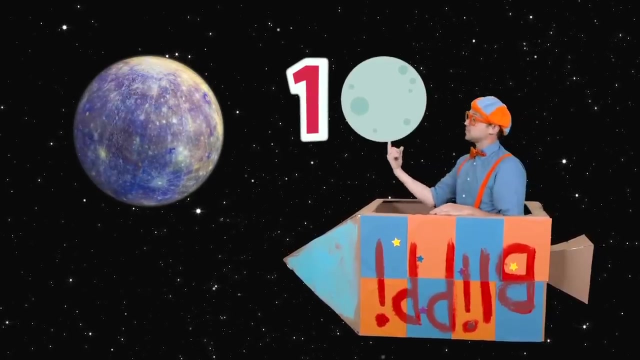 Oh, Look at that planet. That planet is Mercury. Wow, That planet is really rocky And there's so many craters on it And actually, since it's the closest planet to the sun, one rotation around the sun is super fast. It's only about. 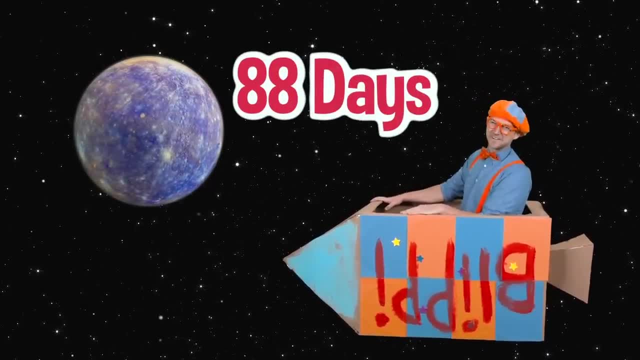 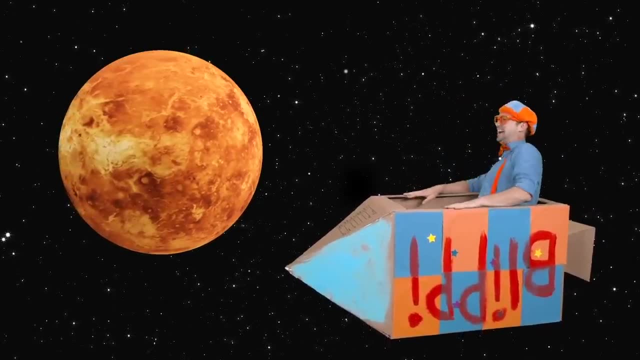 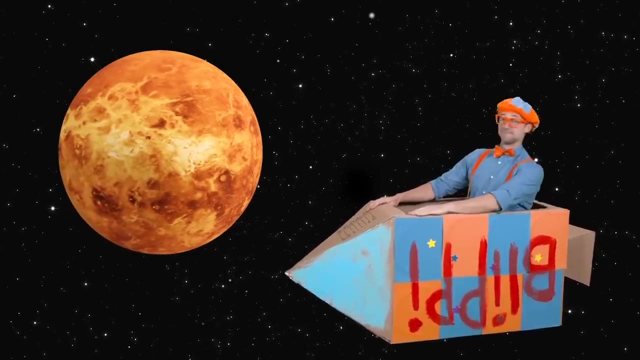 88 days on Earth. Mercury is awesome. Woohoo, Yeah, Woohoo. Now we're at another planet. Look at that planet. That planet is the planet of Venus, And it is so hot, It's the hottest planet. 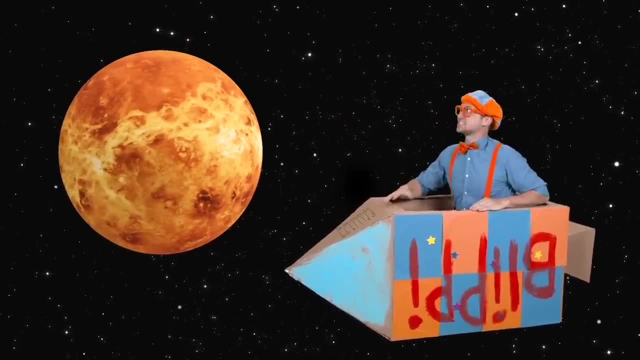 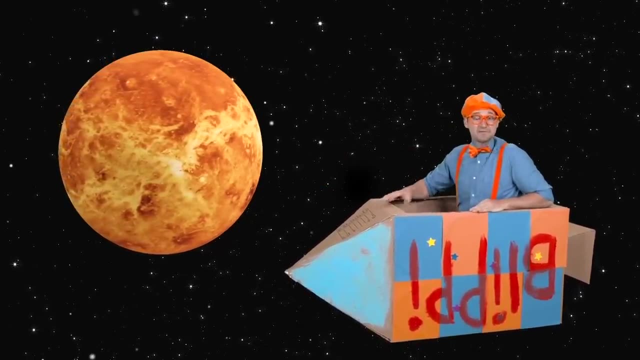 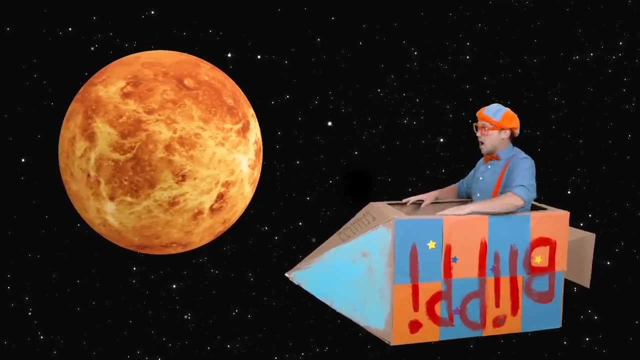 Woo, It's getting hot in here. The planet has so many volcanoes on it And it's actually really bright. If you look up in the sky from our planet Earth, you can actually see it without a telescope. Wow, Here we go. 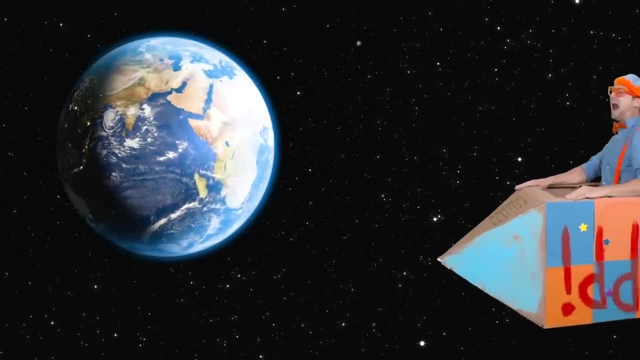 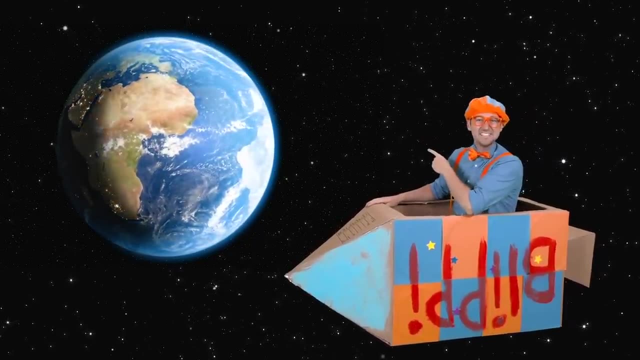 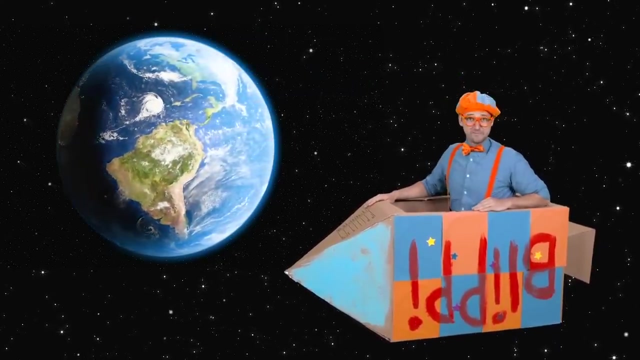 Whoa, Woohoo, This has been awesome. Whoa, Is that you right there? I think I see you. Hey, that's planet Earth. That's where you and I live. Wow, What a beautiful planet. There's so much water. 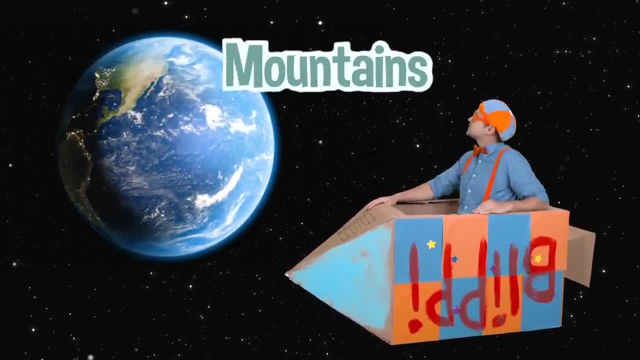 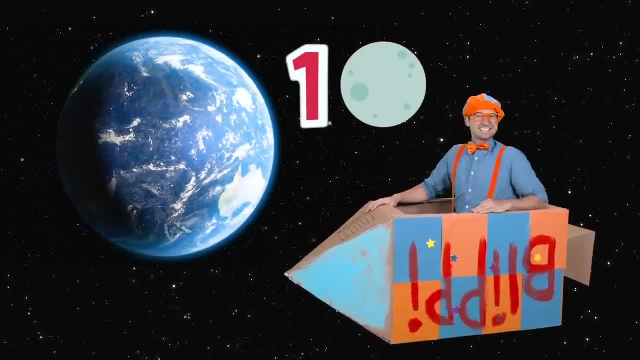 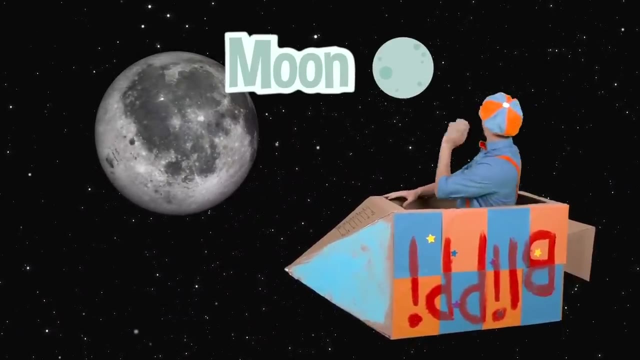 there, And then there's a lot of trees and mountains, Whoa, And our planet Earth. yeah, we have one moon. Let's head there now. Woohoo, Wee, Hey moon. Thank you so much for lighting us up at night. 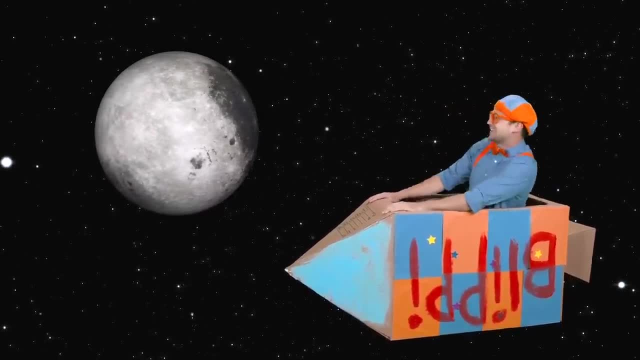 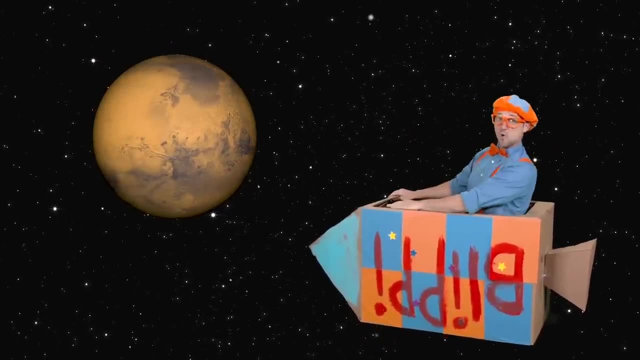 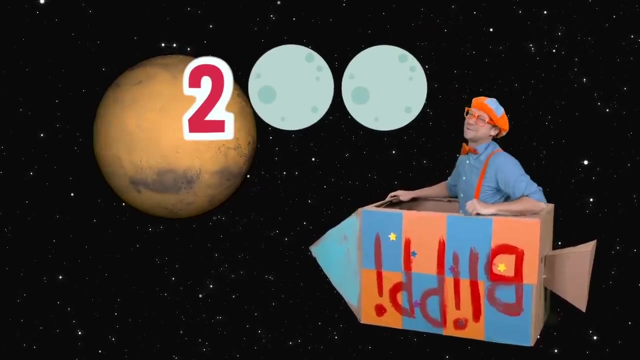 Woohoo, Wee, Woohoo, Another planet. Yeah, Ooh, That planet is the planet Mars. Whoa, It has two moons. Wow, What a lucky planet. Well, we've actually sent robots and rovers to Mars. 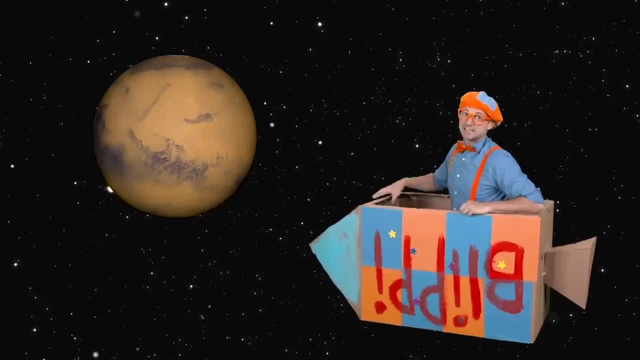 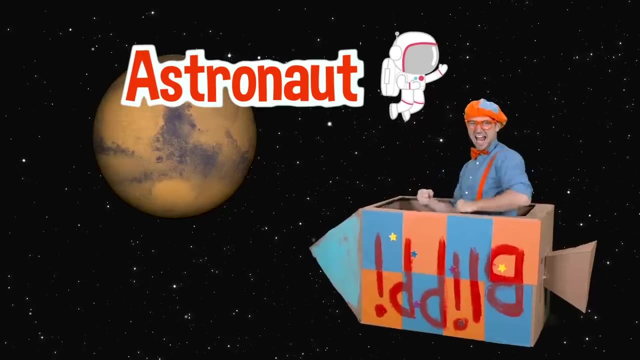 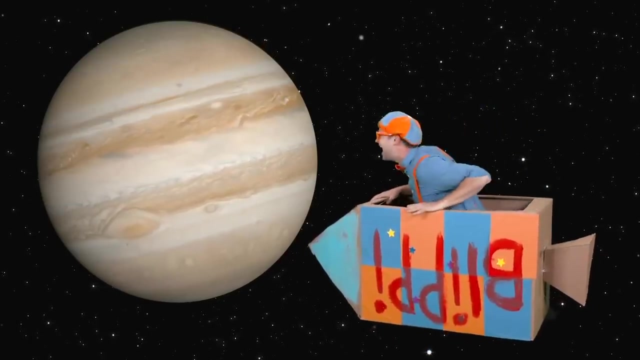 That is awesome. Us humans have yet to land on Mars ourselves, But maybe someday soon, maybe you'll be that astronaut. Yeah, Here we go. Woohoo, Whoa, Haha, That asteroid belt was so intense. Whoa, And look at that. 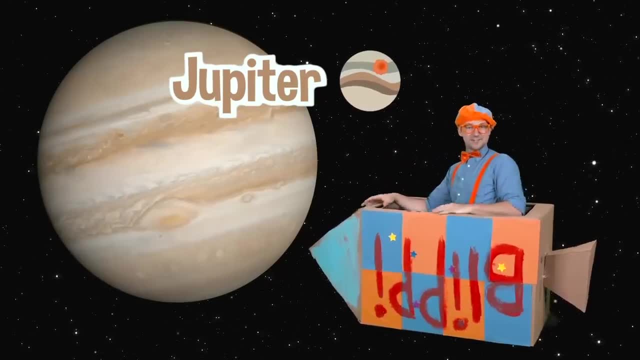 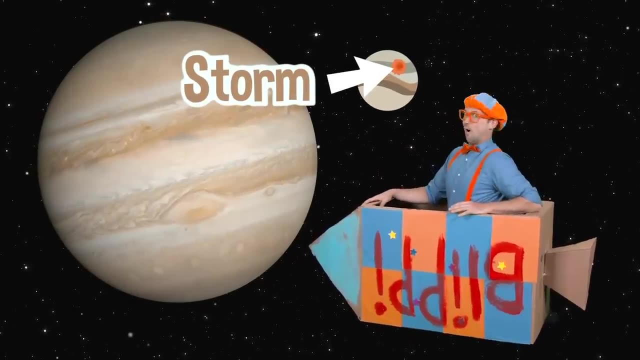 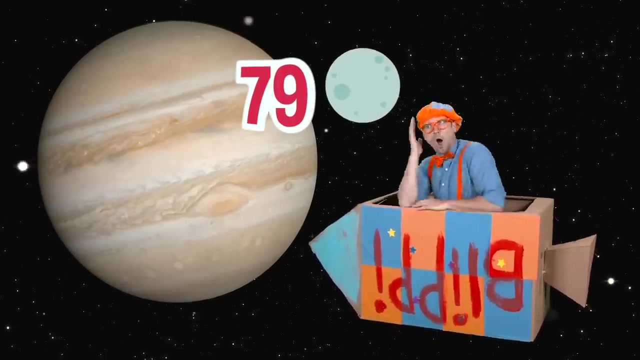 That's our planet, Jupiter. It's the biggest planet in our solar system. And do you see that big red dot? That is a storm. Whoa, That's a big storm. And Jupiter actually has 79 moons. That's crazy. 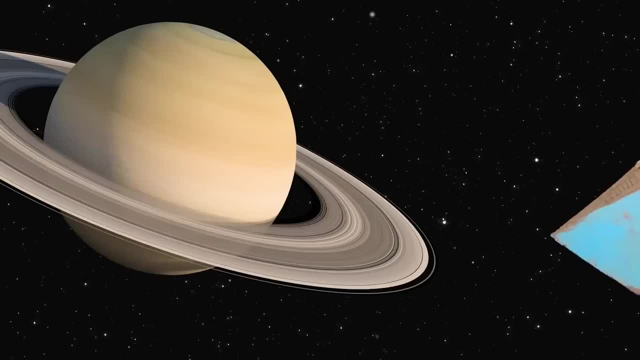 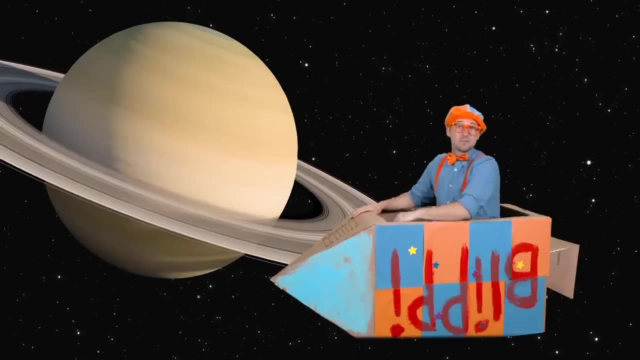 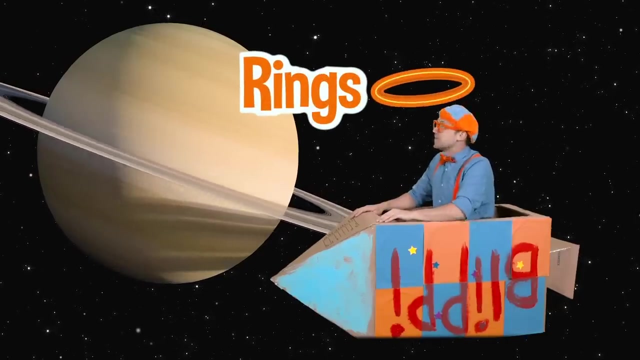 Whoa, Haha, Woohoo, See you later. Jupiter, Hello Saturn, Haha, Check it out. This is our planet, Saturn. Whoa, Look at those. Those are Saturn's rings. Wow, There's so much dust. 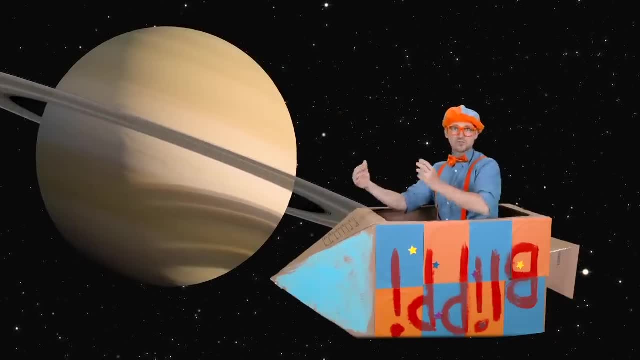 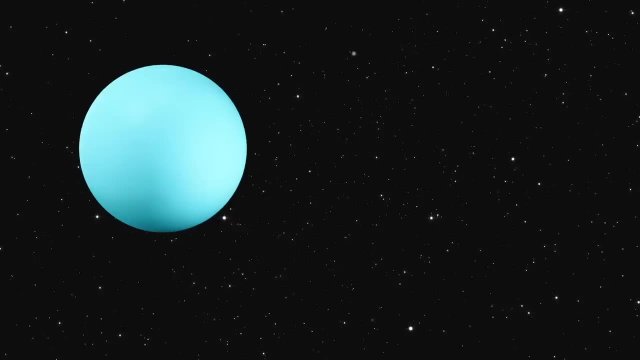 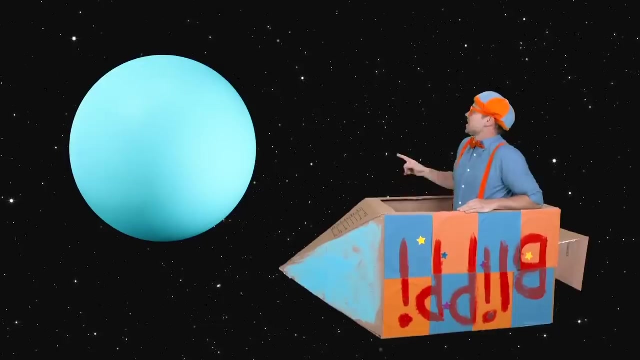 ice and rocks that form those to make up those rings. Wow, What a cool looking planet. Alright, Saturn, See you later. Bye, bye, Haha, Weehee, Haha, Whoa. Oh, look, Another planet, That is Uranus. 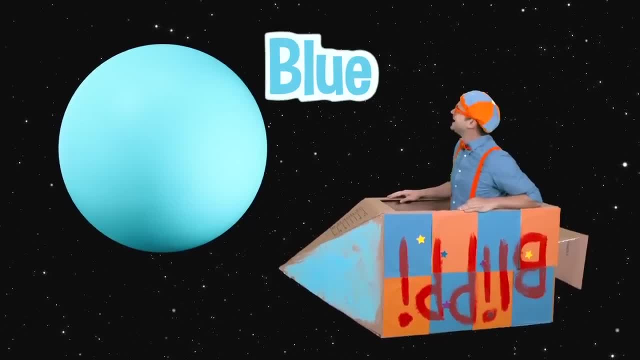 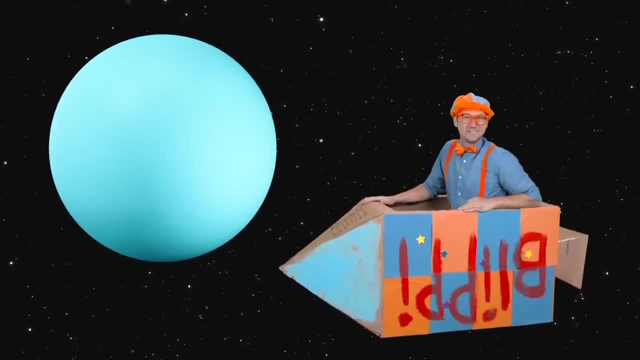 Yeah, What a cool planet, Kind of blue looking, huh, Yeah, That's because there's so much ice on it. It's known as the big ice planet. Whoa, It has 13 rings and 27 moons, Alright. 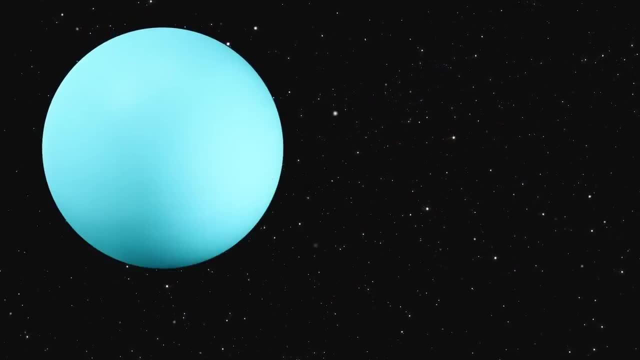 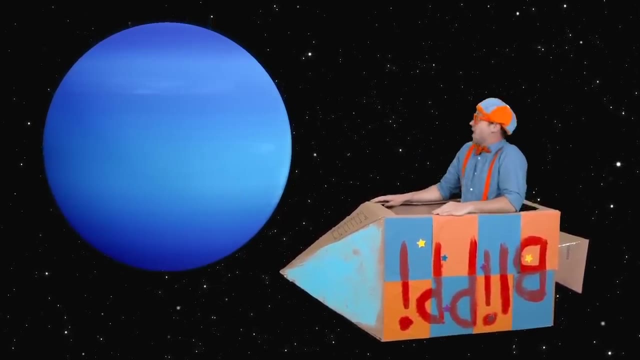 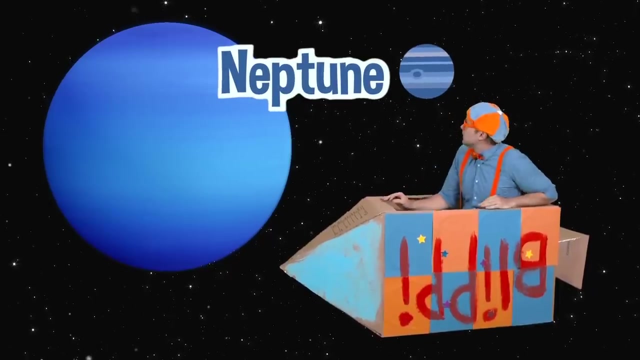 See you later. Uranus, Bye, bye, Whoa. Yeah, This has been so much fun. Whoa, Look at that planet. That planet is the planet Neptune. So dark, cold and windy on that planet. Let's get out. 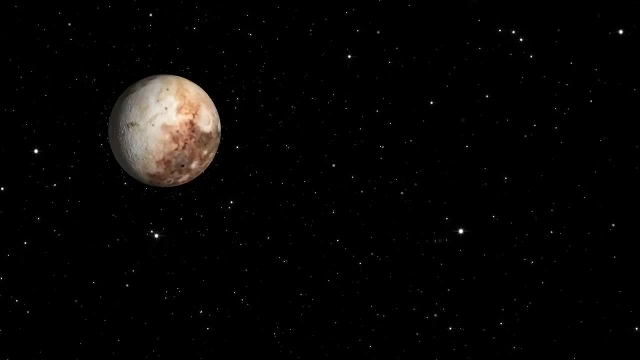 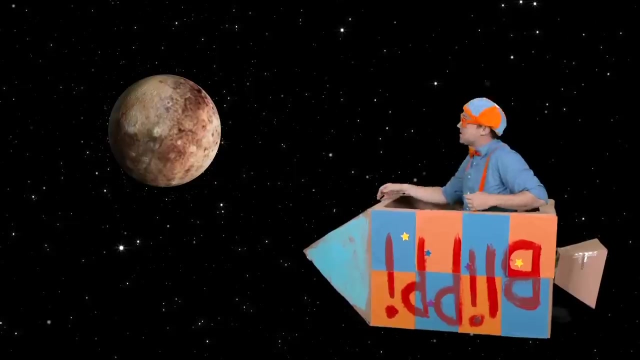 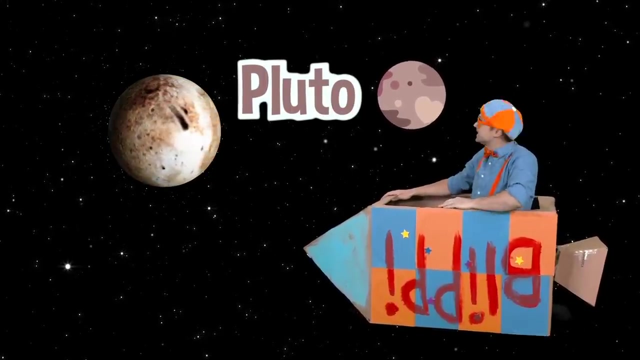 of here. Whoa, Whoa, Woohoo, The last planet on our solar system. Look at it, It's really small. That is Pluto. It's so small, it's a dwarf planet. Wow, And it's really cold. 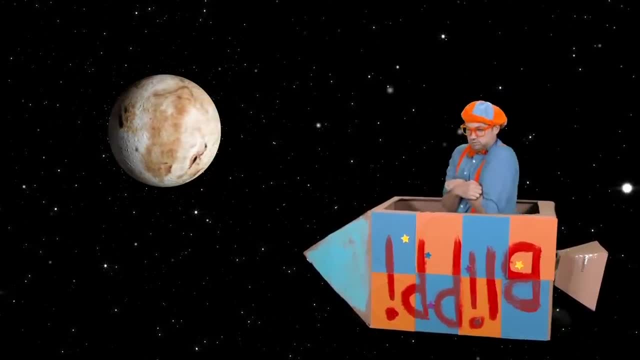 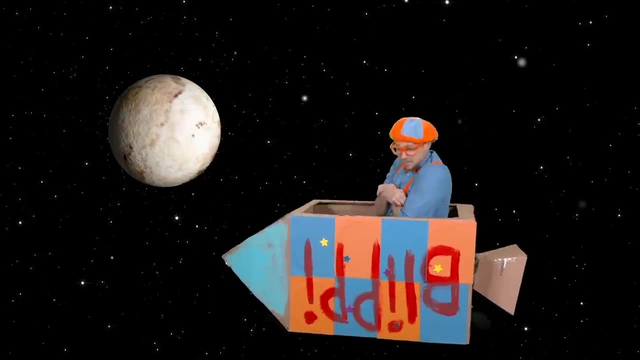 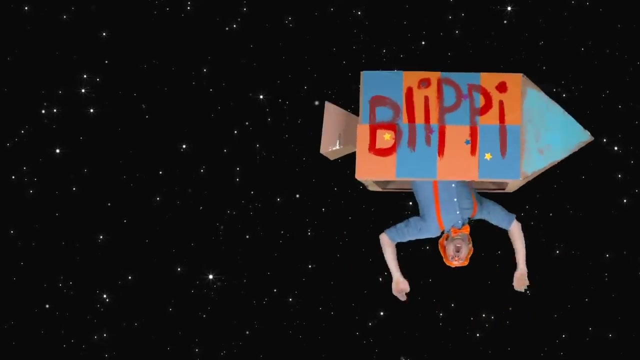 I love Pluto. It's really chilly out here, though. Let's turn around and count all of the planets. Shall we, Woohoo, Yay, Whoa, Whoa. I'm upside down, But now look at my name. 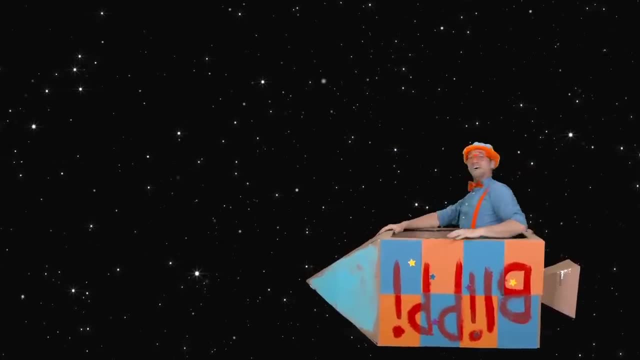 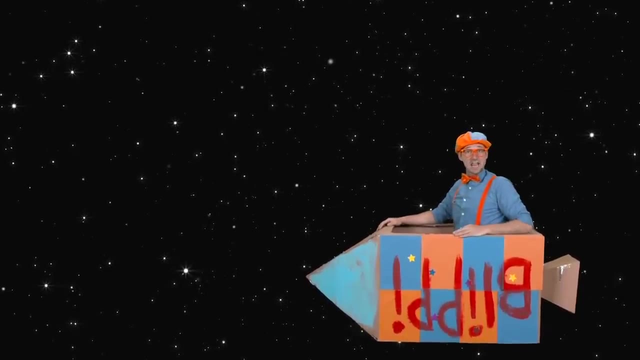 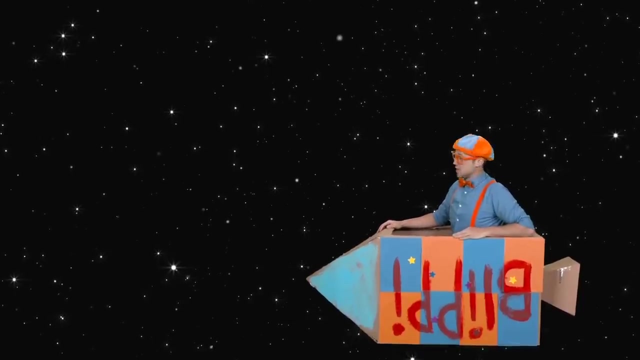 Woohoo, Whoa. That was so much fun learning about all of the planets in our solar system together. Hey, I think we should count all of them. Okay, The sun isn't a planet, So let's count the planets.